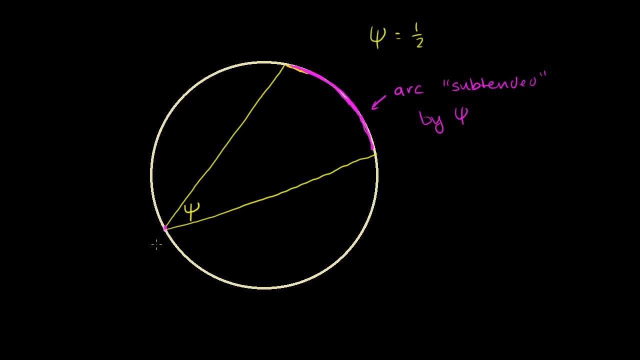 Where psi? is that inscribed angle right over there, the vertex sitting on the circumference? Now, a central angle is an angle where the vertex is sitting at the center of the circle. So let's say that this right here. I'll try to eyeball it. 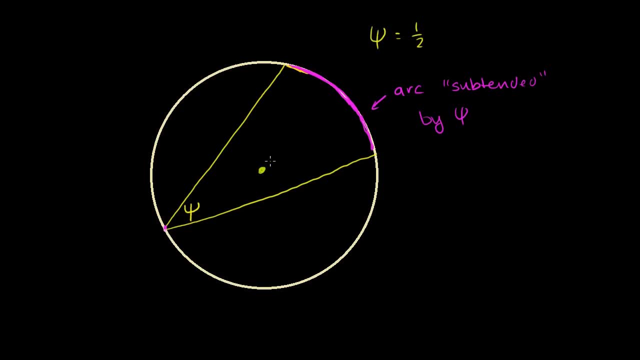 that right there is the center of the circle, And so let me draw a central angle that subtends this same arc. So that looks like a central angle subtending that same arc, Just like that. Let's call this theta, So this angle is psi. 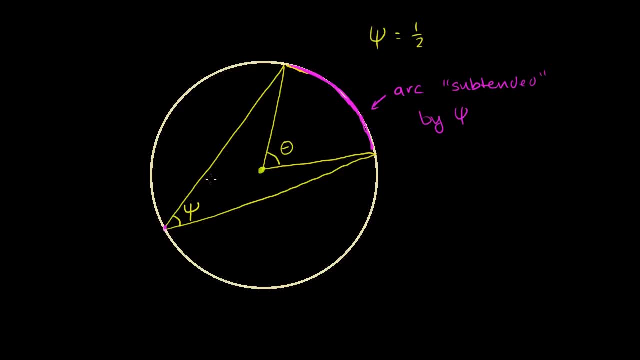 This angle right here is theta, And what I'm going to prove in this video is that psi is always going to be equal to 1 half of theta. So if I were to tell you that psi is equal to, I don't know. 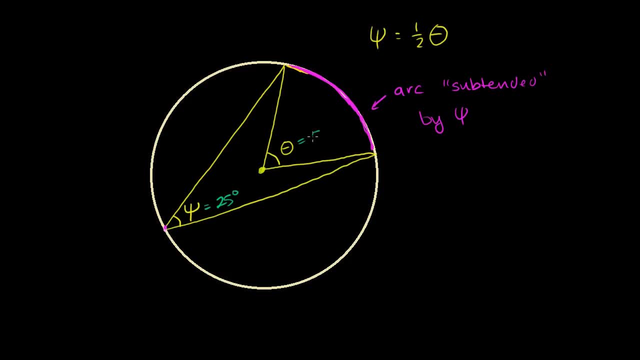 25 degrees, then you would immediately know that theta must be equal to 50 degrees. Or if I told you that theta was 80 degrees, then you would immediately know that theta must be equal to 50 degrees And you would immediately know that psi was 40 degrees. 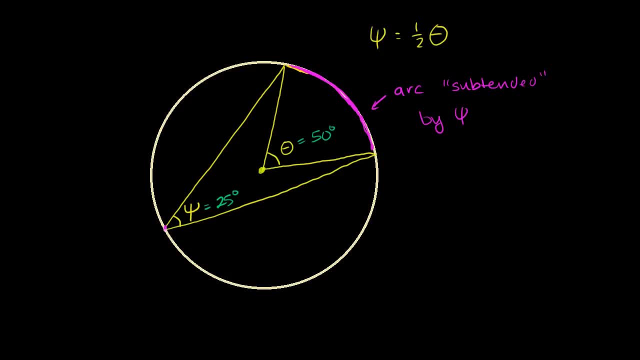 So let's actually prove this. So let me clear this. So a good place to start, or the place I'm going to start, is a special case. I'm going to draw an inscribed angle, But one of the chords that define it is going to be the 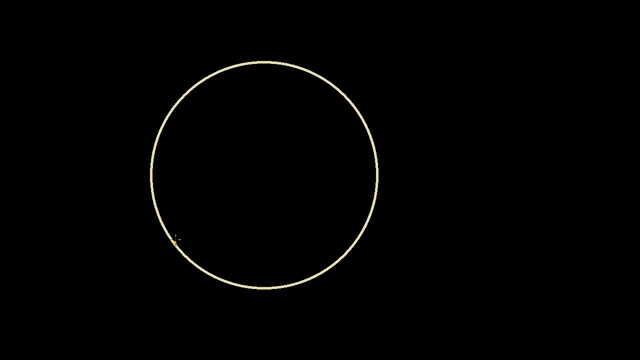 diameter of the circle. So this isn't going to be the general case, This is just going to be a special case. So let me see, This is the center, right here, of my circle. I'm trying to eyeball it. Let me make it a little bit better. 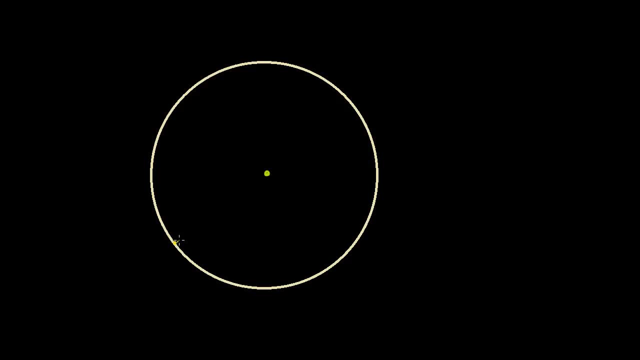 That center looks like that. So let me draw a diameter, So the diameter looks like that, And then let me define my inscribed angle. This diameter is one side of it, And then the other side maybe is just like that. So let me call this right here: psi. 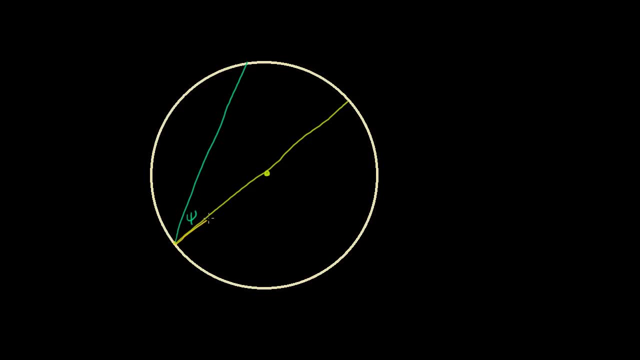 If that's psi, this length right here is a radial. That's our radius of our circle, And then this length right here is also going to be the radius of our circle. We're going from the center to the circumference. The circumference is defined by all of the points that are 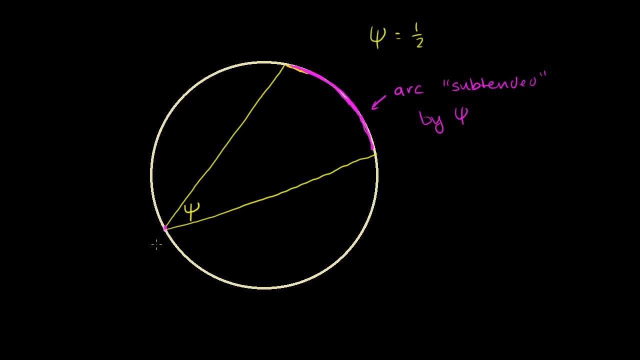 Where psi? is that inscribed angle right over there, the vertex sitting on the circumference? Now, a central angle is an angle where the vertex is sitting at the center of the circle. So let's say that this right here. I'll try to eyeball it. 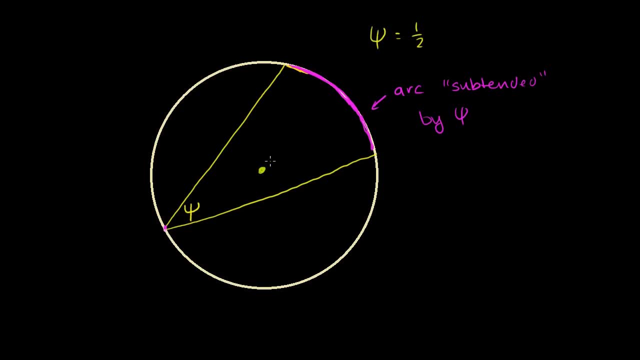 that right there is the center of the circle, And so let me draw a central angle that subtends this same arc. So that looks like a central angle subtending that same arc, Just like that. Let's call this theta, So this angle is psi. 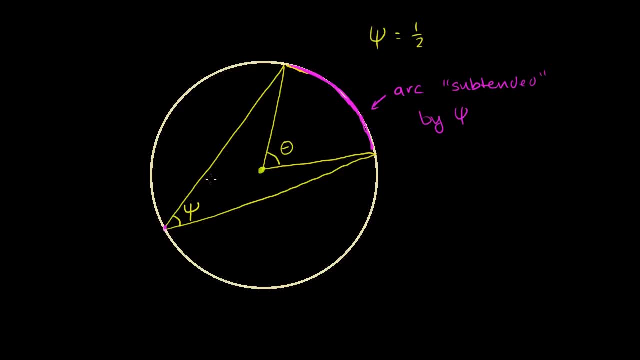 This angle right here is theta, And what I'm going to prove in this video is that psi is always going to be equal to 1 half of theta. So if I were to tell you that psi is equal to, I don't know. 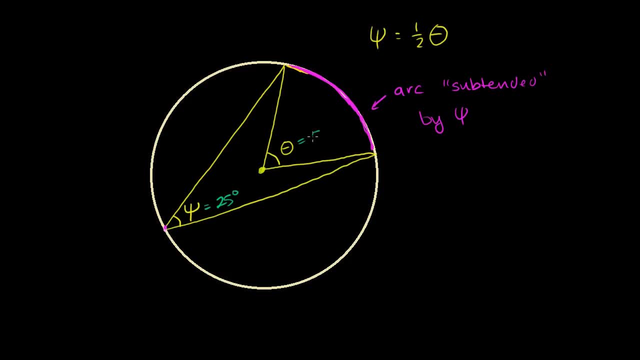 25 degrees, then you would immediately know that theta must be equal to 50 degrees. Or if I told you that theta was 80 degrees, then you would immediately know that theta must be equal to 50 degrees And you would immediately know that psi was 40 degrees. 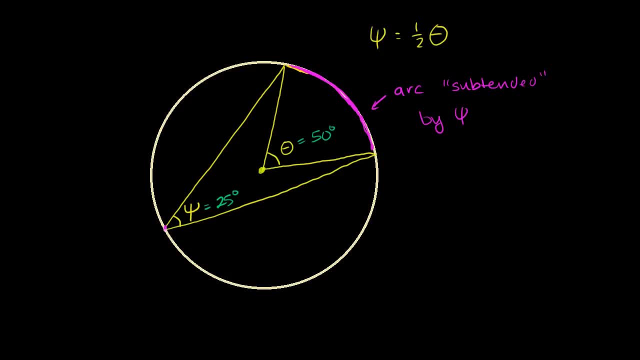 So let's actually prove this. So let me clear this. So a good place to start, or the place I'm going to start, is a special case. I'm going to draw an inscribed angle, But one of the chords that define it is going to be the 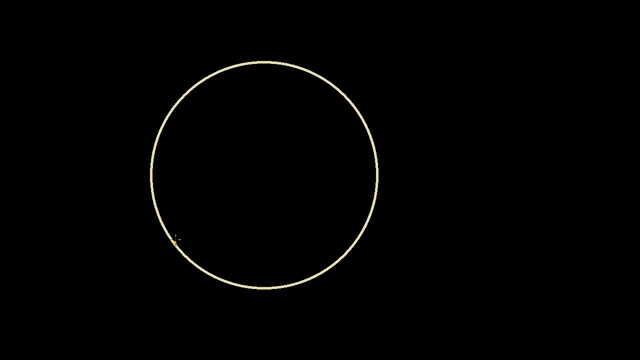 diameter of the circle. So this isn't going to be the general case, This is just going to be a special case. So let me see, This is the center, right here, of my circle. I'm trying to eyeball it. Let me make it a little bit better. 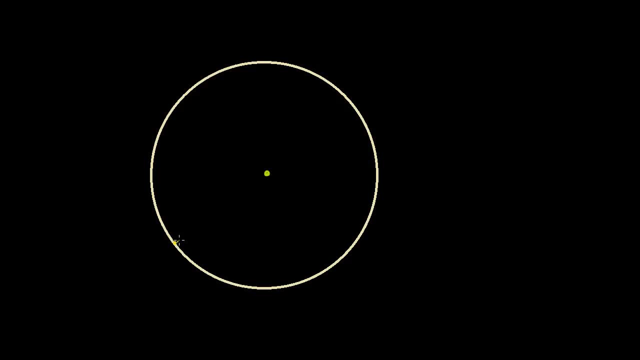 That center looks like that. So let me draw a diameter, So the diameter looks like that, And then let me define my inscribed angle. This diameter is one side of it, And then the other side maybe is just like that. So let me call this right here: psi. 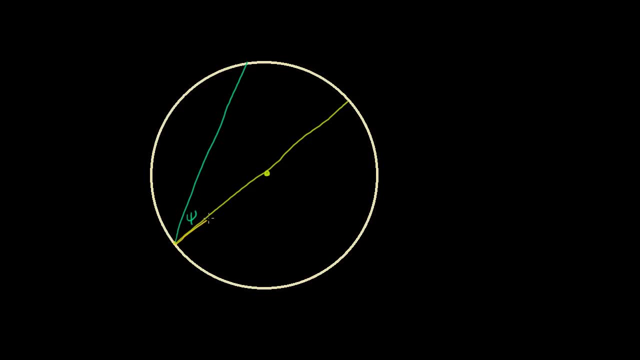 If that's psi, this length right here is a radial. That's our radius of our circle, And then this length right here is also going to be the radius of our circle. We're going from the center to the circumference. The circumference is defined by all of the points that are 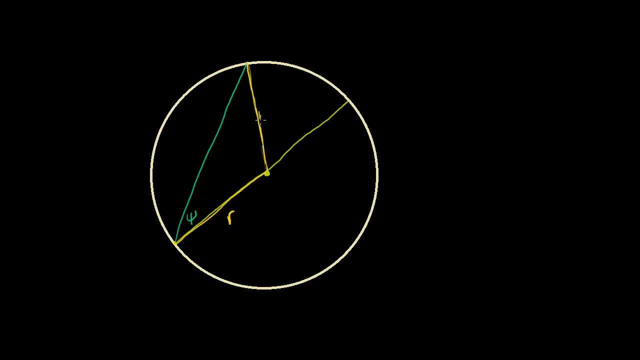 exactly a radius away from the center, So that's also a radius. Now, this triangle right here is an isosceles triangle. It has two sides that are equal, two sides that are definitely equal, And we know that when we have two sides being equal, their 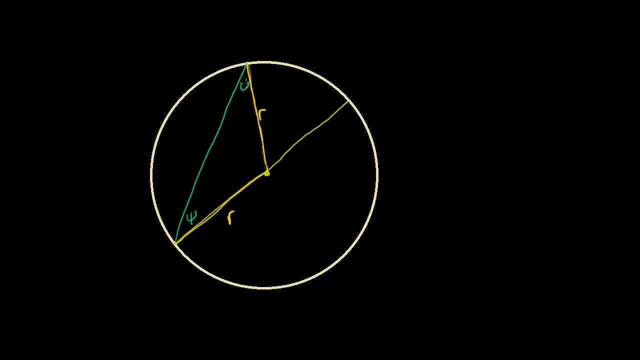 base angles are equal, So this will also be equal to psi. You might not recognize it because it's tilted up like that, But I think many of us, when we see a triangle that looks like this, if I told you this is r and that is r, that these two 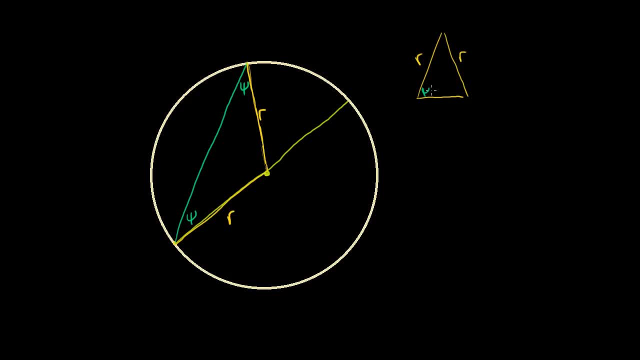 sides are equal, And if this is psi, then you would also know that this angle is also going to be psi. Base angles are equivalent on an isosceles triangle, So if this is psi, that is also equal, So psi. 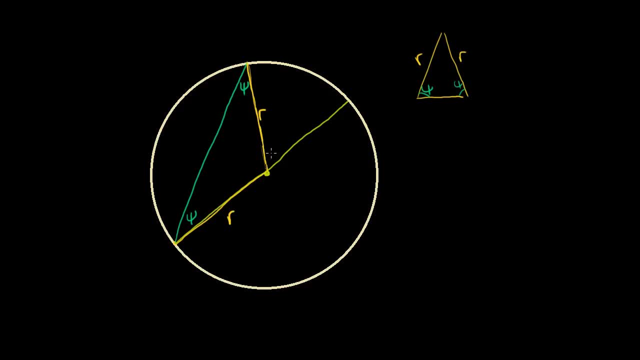 Now let me look at the central angle. This is the central angle subtending the same arc. Let's highlight the arc that they're both subtending. This right here is the arc that they're both going to subtend. So this is my central angle, right there, theta. 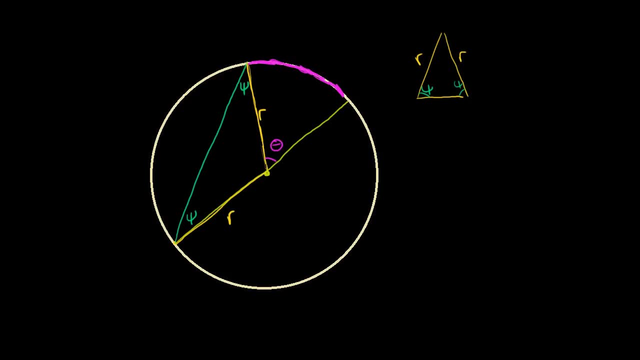 Now, if this angle is theta, what's this angle going to be? This angle right here? Well, this angle is supplementary to theta, So it's 180 minus theta Right. When you add these two angles together, you go 180 degrees. 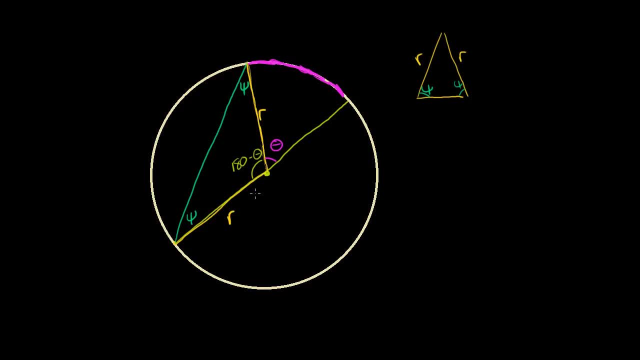 around or they kind of form a line. They're supplementary to each other. Now we also know that these three angles are sitting inside of the same triangle, So they must add up to 180 degrees. So we get psi this, psi plus that, psi plus psi plus this. 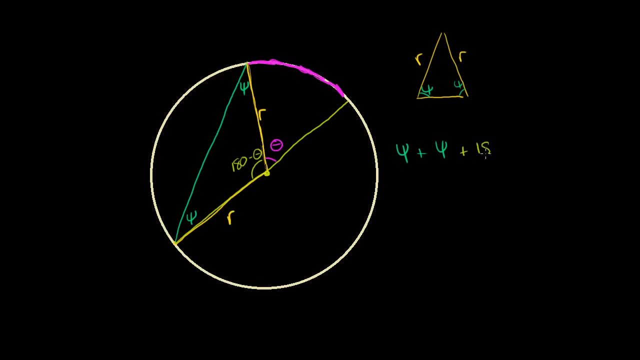 angle which is 180 minus theta plus 180 minus theta. These three angles must add up to 180 degrees. They're the three angles of a triangle. Now we could subtract 180 from both sides. Psi plus psi is 2. psi minus theta is equal to 0.. 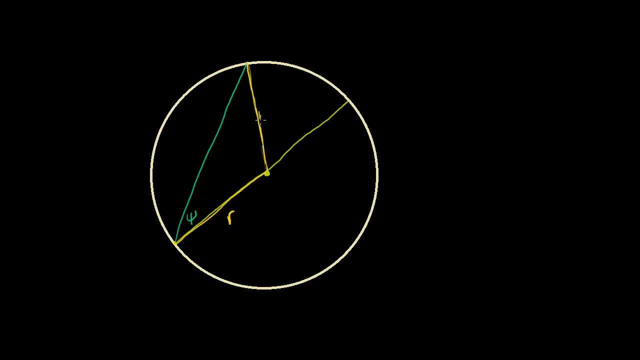 exactly a radius away from the center, So that's also a radius. Now, this triangle right here is an isosceles triangle. It has two sides that are equal, two sides that are definitely equal, And we know that when we have two sides being equal, their 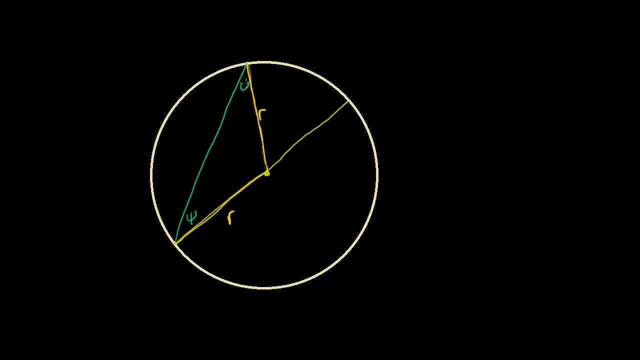 base angles are equal, So this will also be equal to psi. You might not recognize it because it's tilted up like that, But I think many of us, when we see a triangle that looks like this, if I told you this is r and that is r, that these two 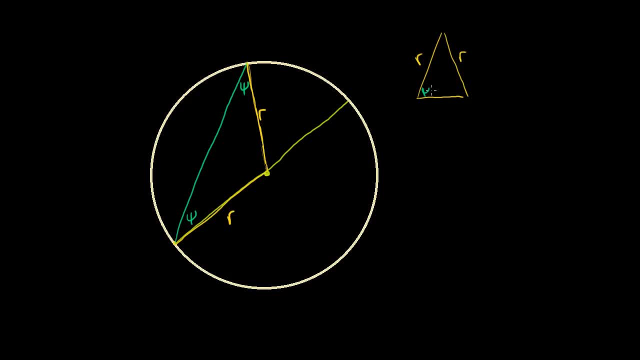 sides are equal, And if this is psi, then you would also know that this angle is also going to be psi. Base angles are equivalent on an isosceles triangle, So if this is psi, that is also equal, So psi. 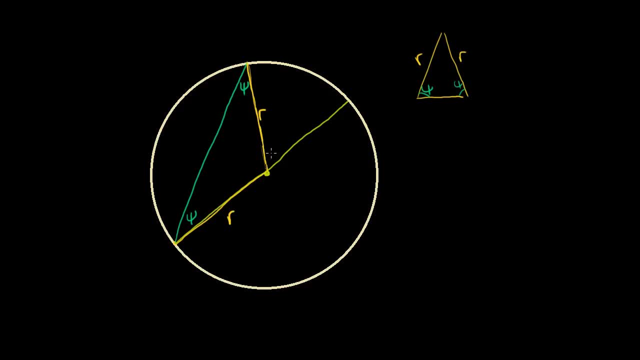 Now let me look at the central angle. This is the central angle subtending the same arc. Let's highlight the arc that they're both subtending. This right here is the arc that they're both going to subtend. So this is my central angle, right there, theta. 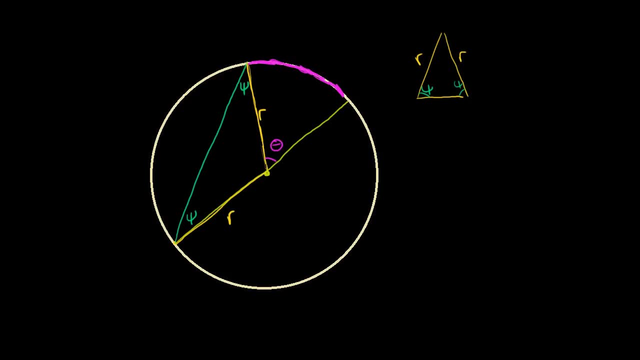 Now, if this angle is theta, what's this angle going to be? This angle right here? Well, this angle is supplementary to theta, So it's 180 minus theta Right. When you add these two angles together, you go 180 degrees. 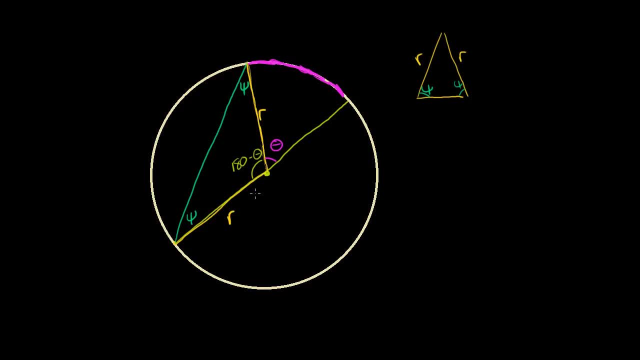 around or they kind of form a line. They're supplementary to each other. Now we also know that these three angles are sitting inside of the same triangle, So they must add up to 180 degrees. So we get psi this, psi plus that, psi plus psi plus this. 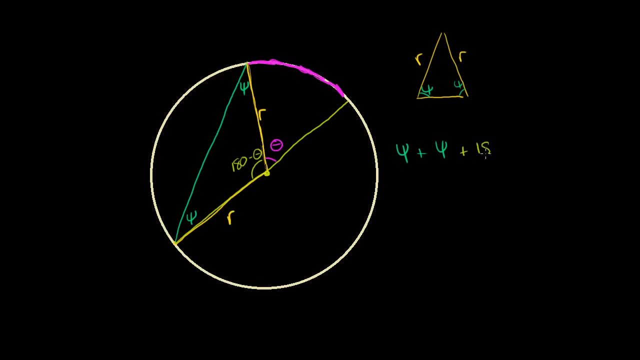 angle which is 180 minus theta plus 180 minus theta. These three angles must add up to 180 degrees. They're the three angles of a triangle. Now we could subtract 180 from both sides. Psi plus psi is 2. psi minus theta is equal to 0.. 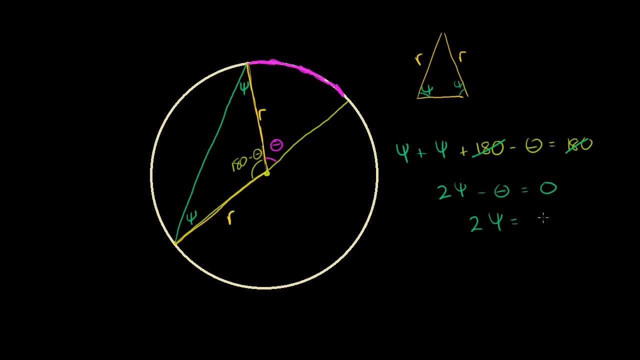 Add theta to both sides, You get 2. psi is equal to theta. Multiply both sides by 1 half or divide both sides by 2. You get psi is equal to 1 half, 1 half of theta. So we just proved what we set out. 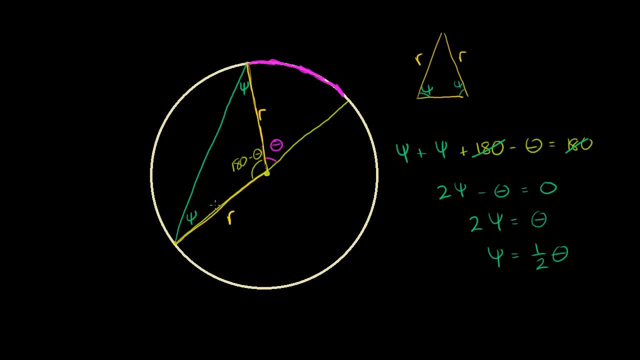 to prove for the special case where our inscribed angle is defined, where one of the rays- if you want to view these lines as rays- where one of the rays that defines this inscribed angle is along the diameter, The diameter forms part of that ray. 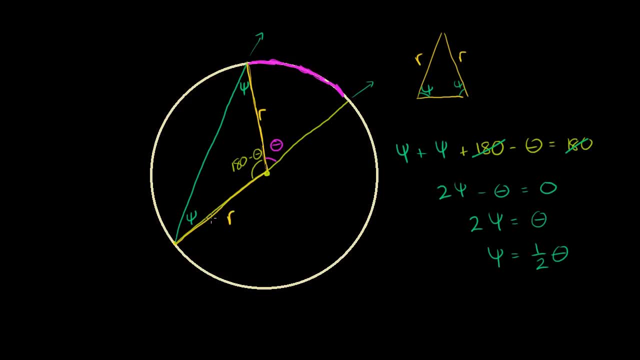 So this is a special case where one edge is sitting on the diameter. So this could apply. So already we could This, We could generalize this. So now that we know that if this is 50, that this is going to be 100 degrees and likewise, 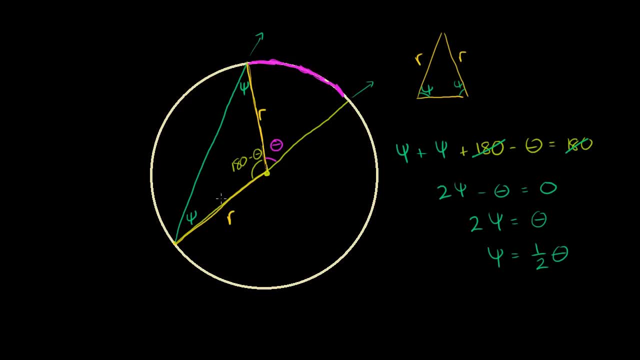 whatever psi is or whatever theta is, psi is going to be 1 half of that. Or whatever psi is, theta is going to be 2 times that. And now this will apply for any time. We can use this notion any time. 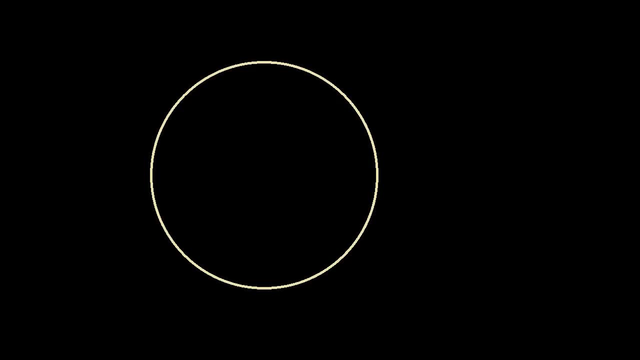 Let me clear this Any time that. So just using that, Using that result we just got, we can now generalize it a little bit, although this won't apply to all inscribed angles. Let's have an inscribed angle that looks like this: 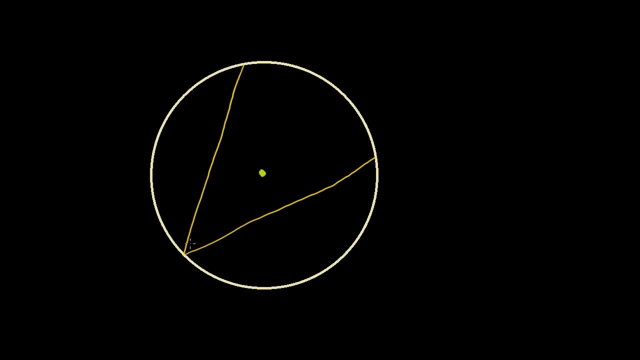 So in this situation, the center, you can kind of view it as it's inside of the angle, That's my inscribed angle, And I want to find a relationship between this inscribed angle and the central angle that's subtending the same arc. 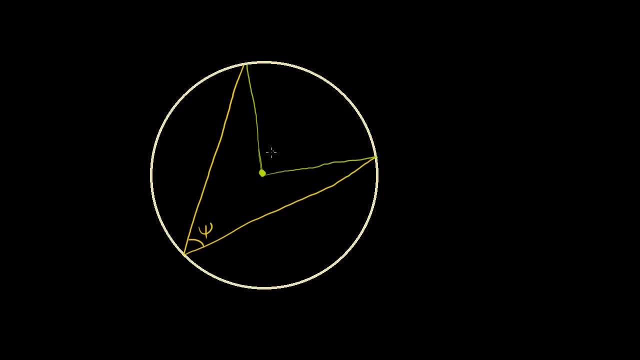 My central angle subtending the same arc. Well, you might say, hey gee, none of these ends or these chords that define this angle. neither of these are diameters. But what we can do is we can draw a diameter If the center is within these two chords. 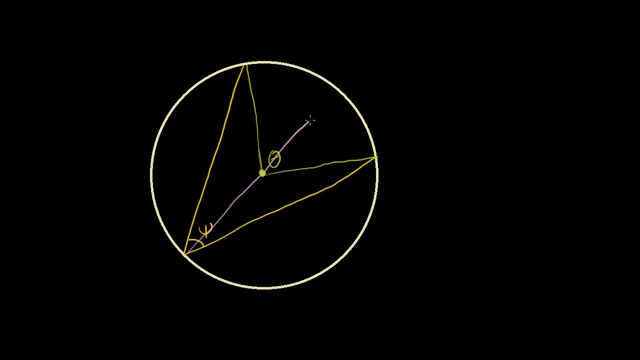 we can draw a diameter. We can draw a diameter just like that. If we draw a diameter, just like that, if we define this angle as psi 1, that angle as psi 2,, clearly psi is the sum of those two angles. 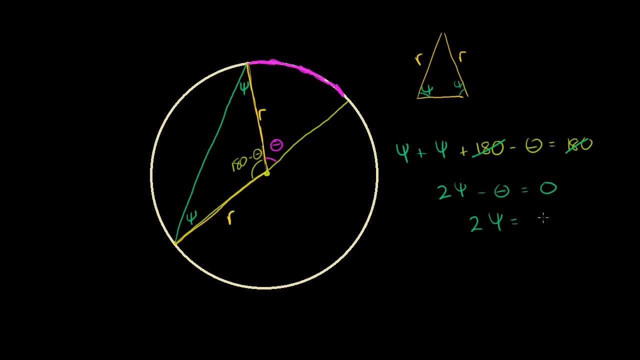 Add theta to both sides, You get 2. psi is equal to theta. Multiply both sides by 1 half or divide both sides by 2. You get psi is equal to 1 half, 1 half of theta. So we just proved what we set out. 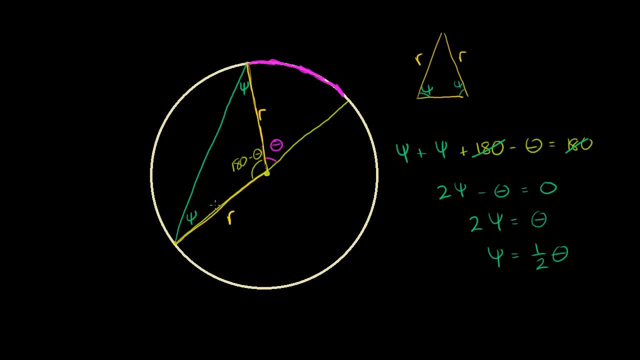 to prove for the special case where our inscribed angle is defined, where one of the rays- if you want to view these lines as rays- where one of the rays that defines this inscribed angle is along the diameter, or the diameter forms part of that ray. 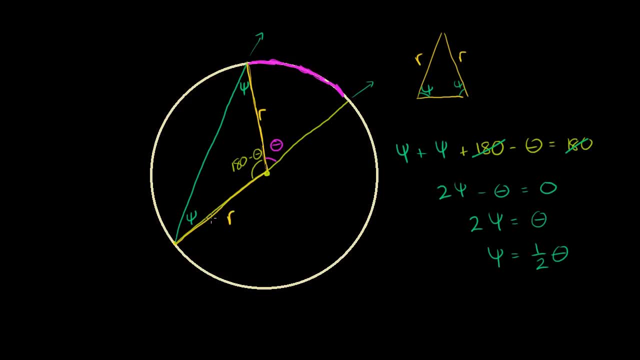 So this is a special case where one edge is sitting on the diameter. So this could apply. So already we could This, We could generalize this. So now that we know that if this is 50, that this is going to be 100 degrees and likewise, 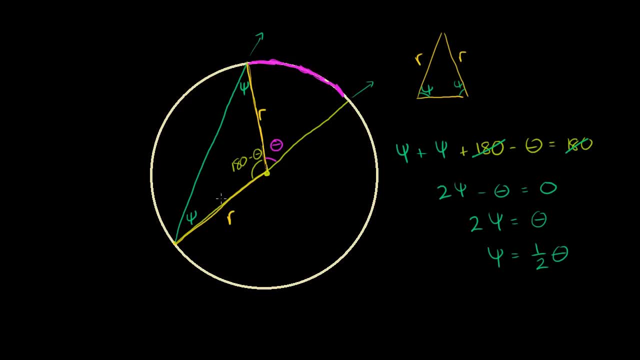 whatever psi is or whatever theta is, psi is going to be 1 half of that. Or whatever psi is, theta is going to be 2 times that. And now this will apply for any time. We can use this notion any time. 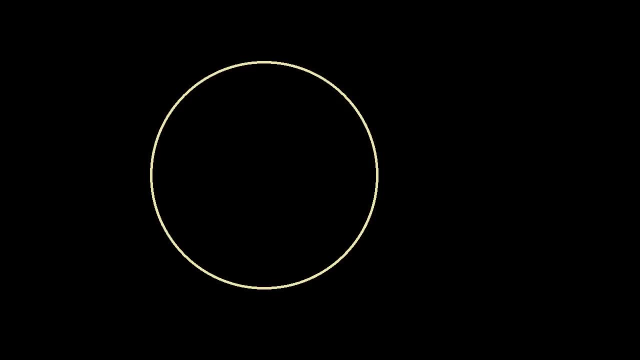 Let me clear this Any time that. So, just using that, Using that result we just got, we can now generalize it a little bit, Although this won't apply to all inscribed angles. Let's have an inscribed angle that looks like this: 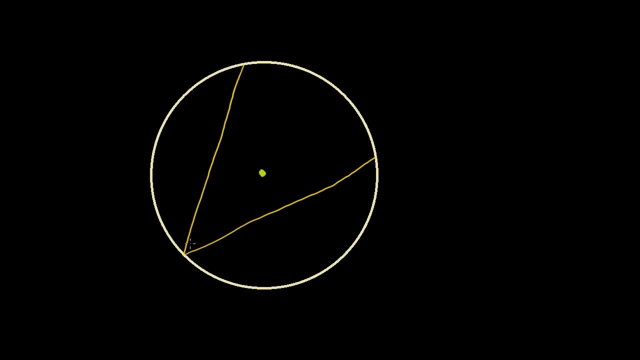 So in this situation, the center, you can kind of view it as it's inside of the angle, That's my inscribed angle, And I want to find a relationship between this inscribed angle and the central angle that's subtending the same arc. 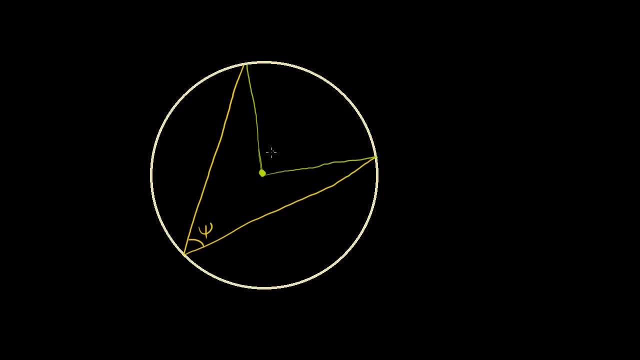 My central angle subtending the same arc. Well, you might say, hey gee, none of these ends or these chords that define this angle. neither of these are diameters. but what we can do is we can draw a diameter If the center is within these two chords. 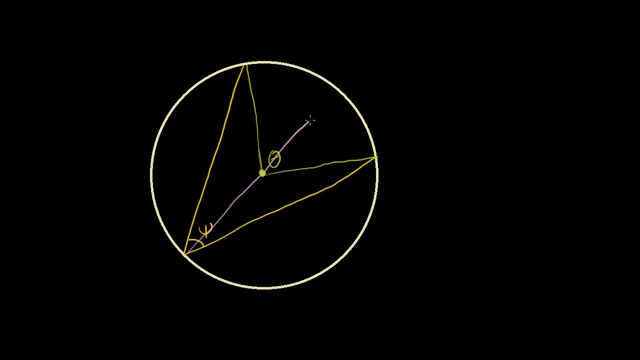 we can draw a diameter. We can draw a diameter just like that. If we draw a diameter, just like that, if we define this angle as psi, 1. That angle as psi, 2. Clearly, psi is the sum of those two angles. 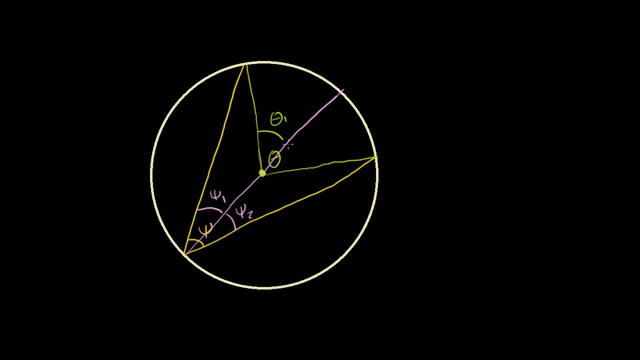 And we call this angle theta 1 and this angle theta 2.. We immediately know that, just using the result I just got, since we have one side of our angles in both cases being a diameter, now we know that psi 1 is going to be equal to 1. 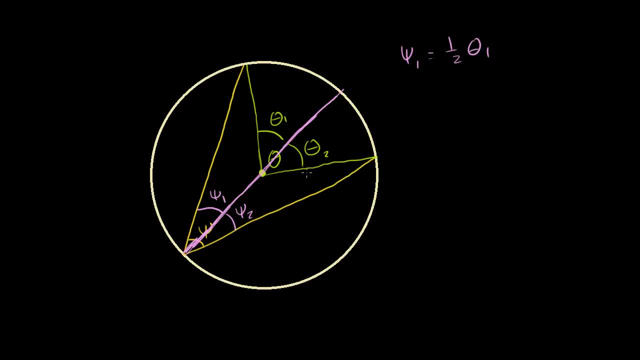 half theta 1.. And we know that psi 2 is going to be 1 half theta 2.. Psi, Psi 2 is going to be 1 half theta 2.. And so psi, which is psi 1 plus psi 2.. 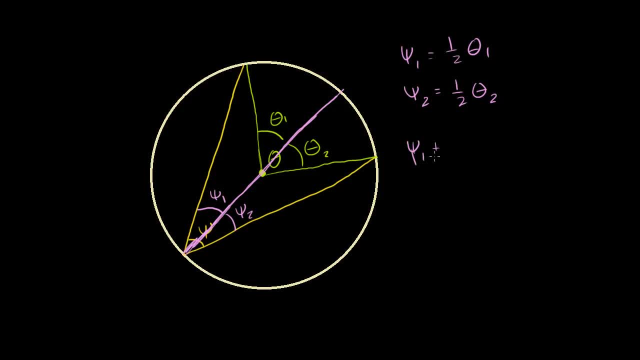 So psi 1 plus- let me write the psi a little better: Psi 1 plus psi 2 is going to be equal to these two things: 1 half theta 1 plus 1 half theta 2.. Psi 1 plus psi 2, this is equal to the first inscribed angle. 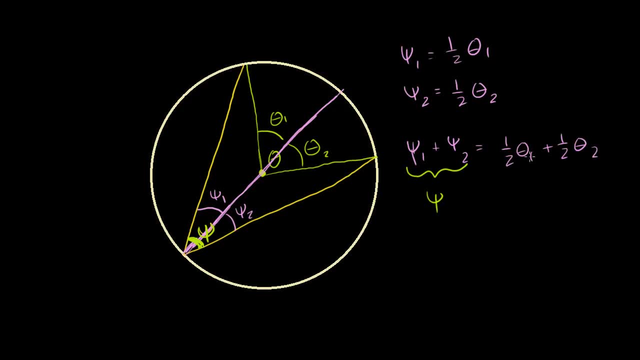 that we want to deal with just regular psi. That's psi And this right here. this is equal to 1 half times theta 1 plus theta 2.. What's theta 1 plus theta 2?? Well, that's just our original theta that we were dealing. 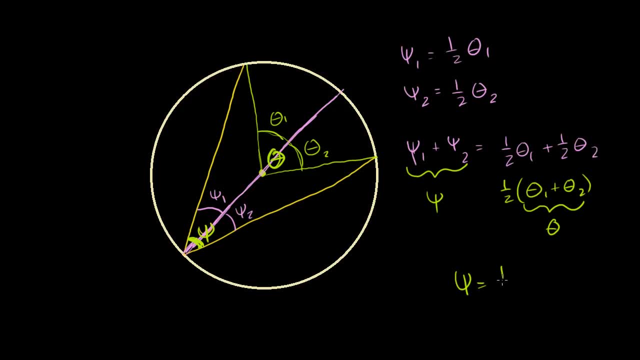 with our original theta. So now we see that psi is equal to 1 half theta. So now we've proved it for a slightly more general case, where our center is inside of the two rays that define that angle. Now we still haven't addressed a. 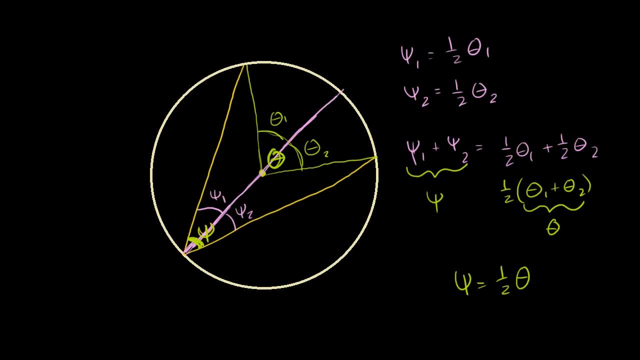 slightly harder situation or a more general situation where, if this is the center of our circle and I have an inscribed angle where the center isn't sitting inside of the two chords, So let me draw that. So let's say I have that's going to be my vertex. 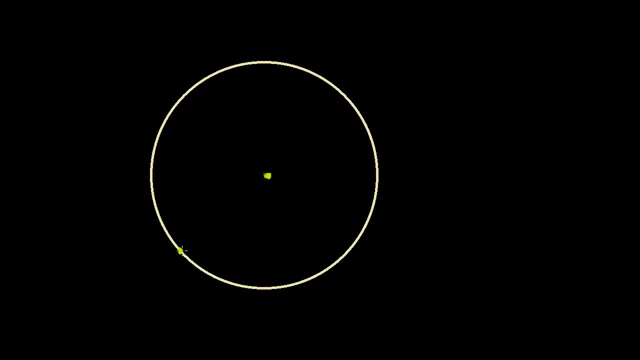 And I'll switch colors. So let's say that is one of the chords that defines the angle, just like that. And let's say that is the other chord that defines the angle, just like that. So how do we find the relationship between let's. 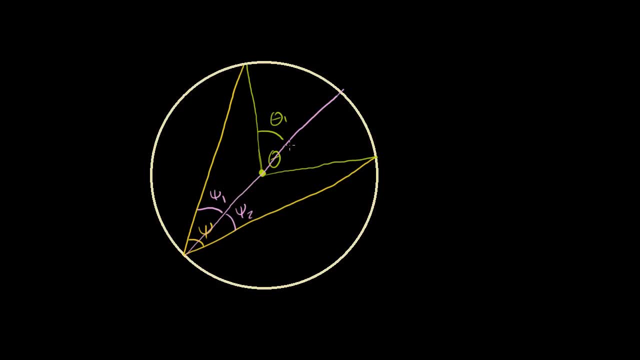 and we call this angle theta 1 and this angle theta 2, we immediately know that, just using the result I just got, since we have one side of our angles in both cases being a diameter, now we know that psi 1 is going to be equal. 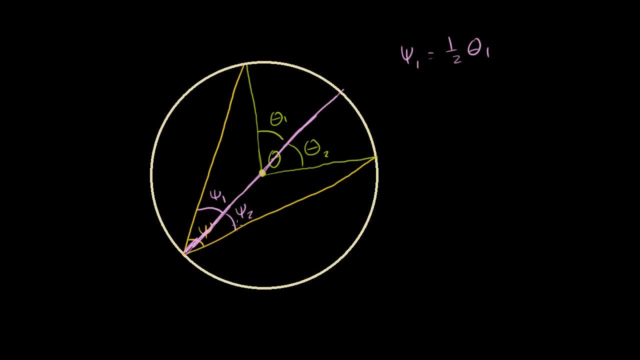 to 1 half theta 1.. And we know that psi 2 is going to be 1 half theta 2.. Psi, Psi 2, is going to be 1 half theta 2.. And so psi, which is psi 1 plus psi 2, so psi 1 plus. 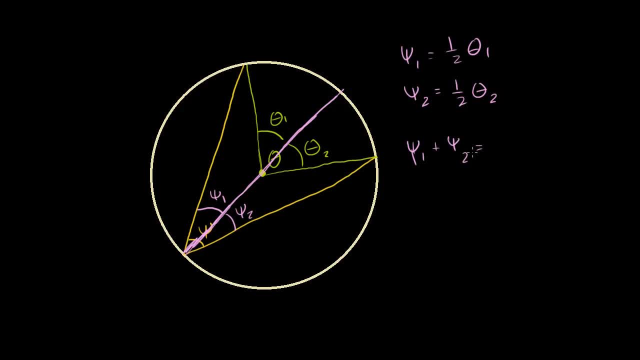 let me write the psi a little better. psi 1 plus psi 2 is going to be equal to these two things: 1 half theta 1 plus 1 half theta 2.. Psi 1 plus psi 2, this is equal to the first inscribed angle. 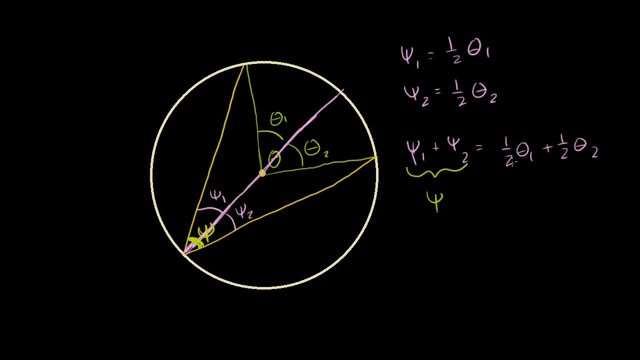 that we want to deal with just regular psi. That's psi And this right here. this is equal to 1 half times theta 1 plus theta 2.. What's theta 1 plus theta 2?? Well, that's just our original theta that we were dealing with. 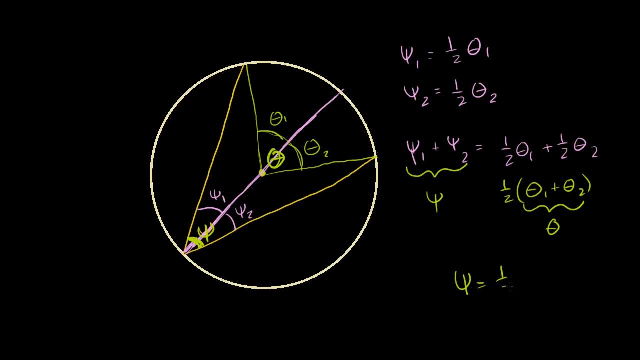 our original theta. So now we see that psi is equal to 1 half theta. So now we've proved it for a slightly more general case, where our center is inside of the two rays that define that angle. Now we still haven't addressed a solution. 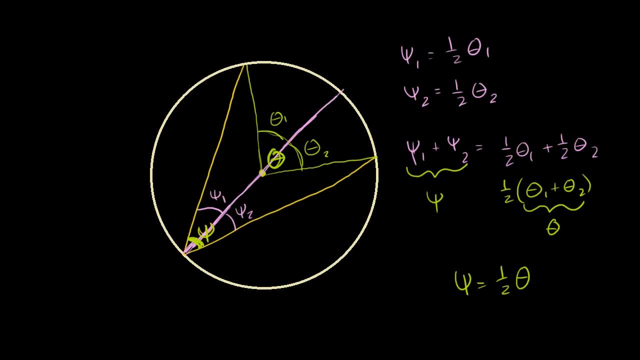 A slightly harder situation or a more general situation where, if this is the center of our circle and I have an inscribed angle where the center isn't sitting inside of the two chords, So let me draw that. So let's say I have, that's going to be my vertex. 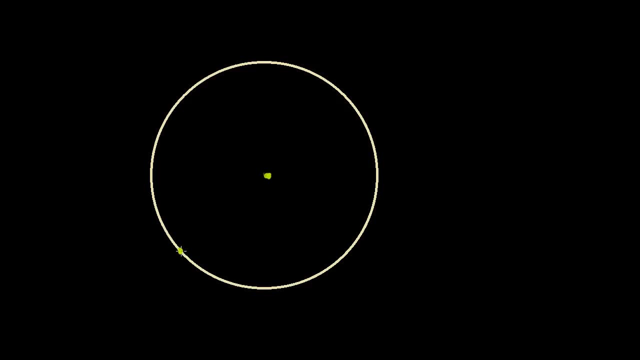 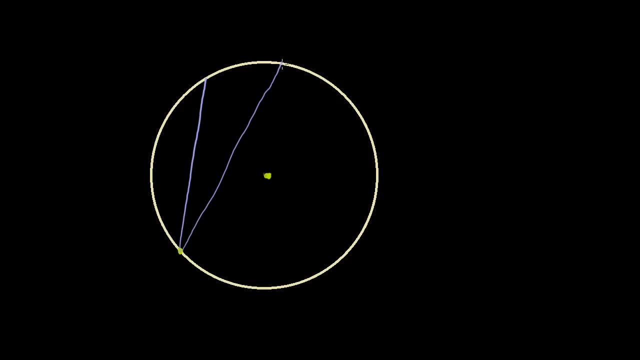 And let's say that is the other angle, And let's say that is the other chord. that defines the angle, just like that. So how do we find the relationship between, let's call this angle right here, let's call it psi 1.. 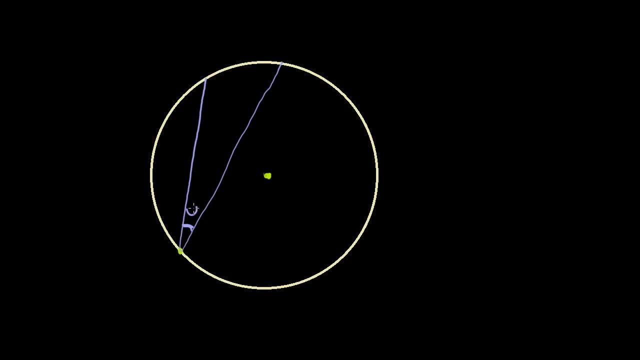 call this angle right here. let's call it psi 1.. How do we find the relationship between psi 1 and the central angle that subtends this same arc? So when I talk about the same arc, that's that right there. So the central angle that subtends the same arc will. 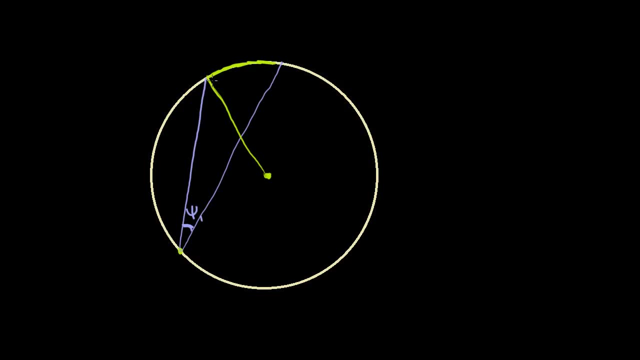 look like this. It will look like this. Let's call that theta 1.. What we could do is use what we just learned when one side of our inscribed angle is a diameter. So let's construct that. So let me draw a diameter here. 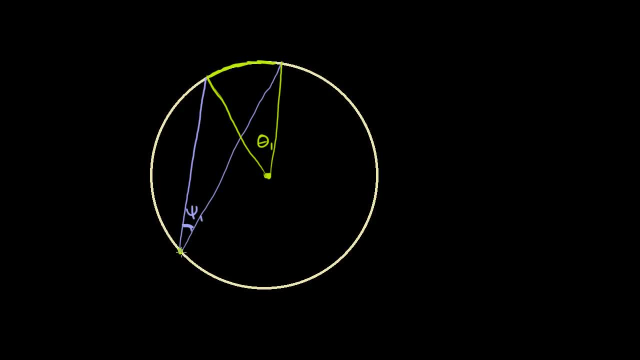 The result we want still is that this should be one half of this. But let's prove it. Let's draw a diameter. let's draw a straighter diameter than that. So let's draw a diameter. Let's draw a diameter just like that. 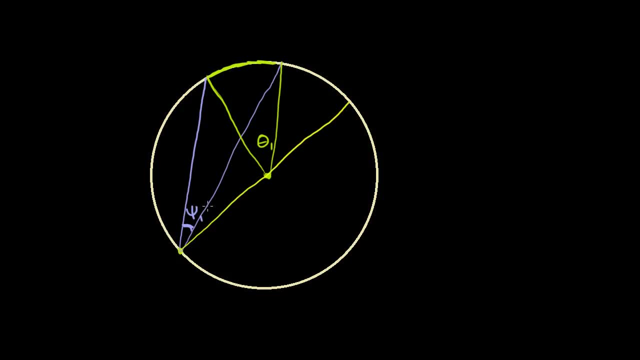 And let me call this angle right here, this angle right there. let me call that psi 2.. Let me call that psi 2.. And it is subtending this angle, this arc, right there. Let me do that in a darker color. 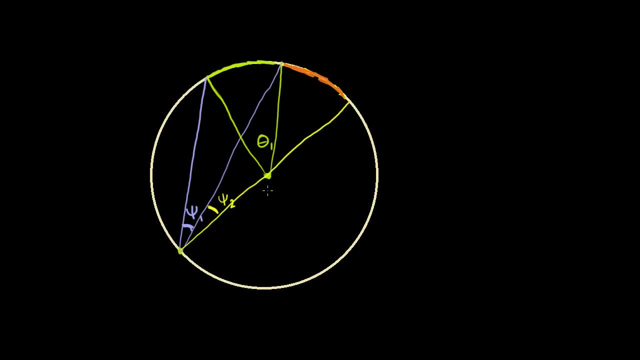 It is subtending this arc right there, And so the central angle that subtends that same arc. let me call that theta 2.. Now we know from the last, from really just the earlier part of this video, that psi 2 is going to be equal to one. 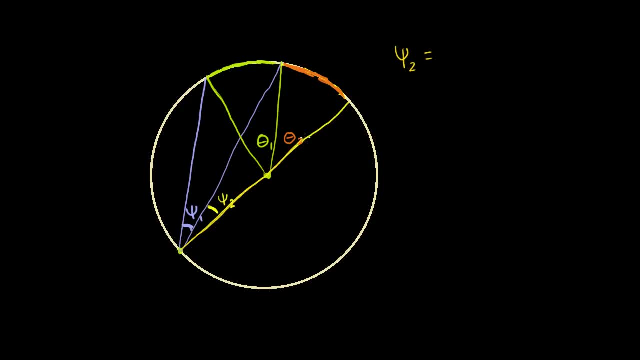 half theta 2, right, They share. the diameter is right there. The diameter is one of the chords that forms the angle. So psi 2 is going to be equal to one half theta 2.. This is exactly what we've been doing in the last video. 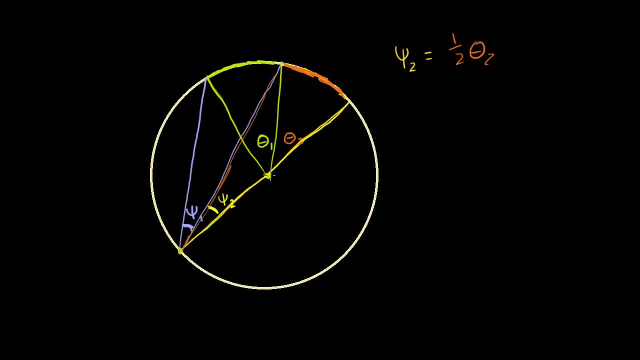 right. This is an inscribed angle. This is an inscribed angle. One of the chords that define it is sitting on the diameter, So this is going to be one half of this angle, of the central angle that subtends the same arc. 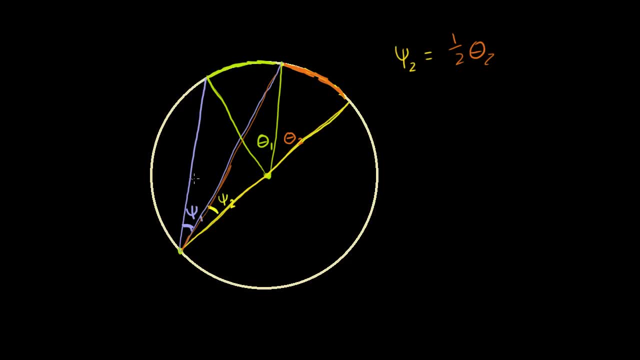 Now let's look at this larger angle. This larger angle right here: Psi 1 plus psi 2, right, That larger angle is psi 1 plus psi 2.. Once again, This subtends this entire arc right here. So it's going to be, and it has a diameter as one of the chords. 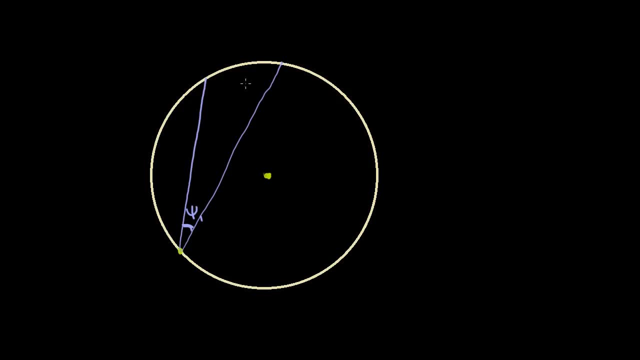 How do we find the relationship between psi 1 and the central angle that subtends this same arc? So when I talk about the same arc, that's that right there. So the central angle that subtends the same arc will look like this: 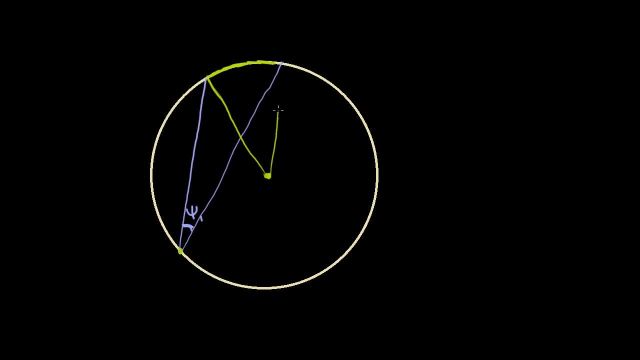 It will look like this: Let's call that theta 1.. What we could do is use what we just learned when one side of our inscribed angle is a diameter. So let's construct that. So let me draw a diameter here. The result we want still is that this should be 1 half of. 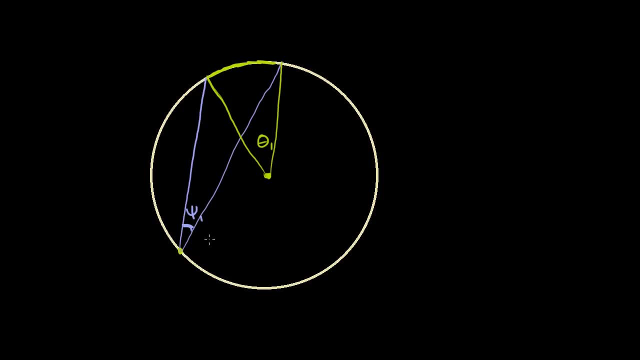 this, but let's prove it. Let's draw a diameter. Let's draw a straighter diameter than that. So let's draw, Let's draw a diameter, just like that. And let me call this angle right here, this angle right there. 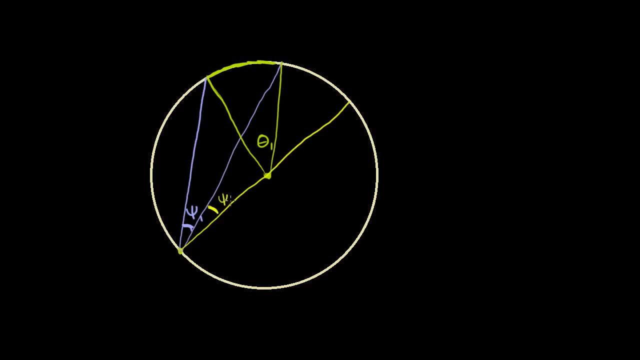 let me call that psi 2.. And it is subtending this angle, this arc right there. Let me do that in a darker color. It is subtending this arc right there, And so the central angle that subtends that same arc. 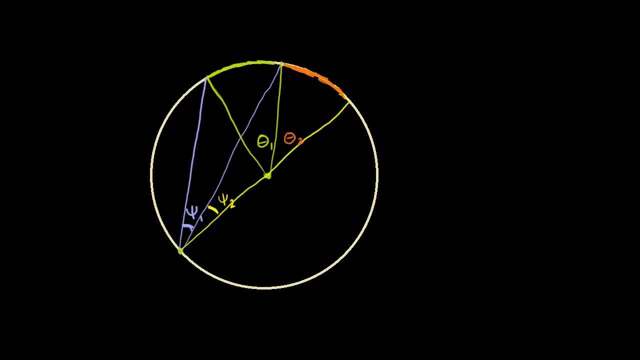 let me call that theta 2.. Now we know from the last, from really just the earlier part of this video, that psi 2 is going to be equal to 1, half theta 2, right, They share. the diameter is right there. 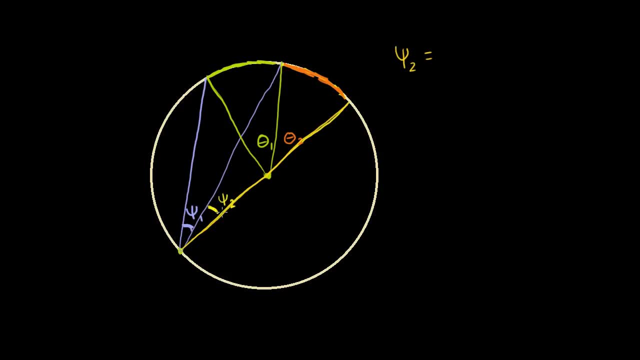 The diameter is one of the chords that forms the angle. So psi 2 is going to be equal to 1, half theta 2.. This is exactly what we've been doing in the last video. right, This is an inscribed angle. 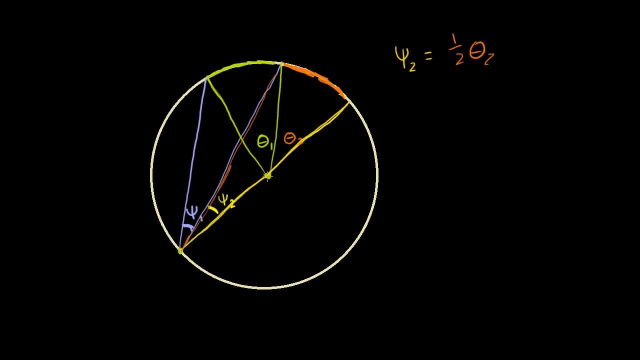 Let's draw a diameter. One of the chords that define it is sitting on the diameter, So this is going to be 1 half of this angle, of the central angle that subtends the same arc. Now let's look at this larger angle. 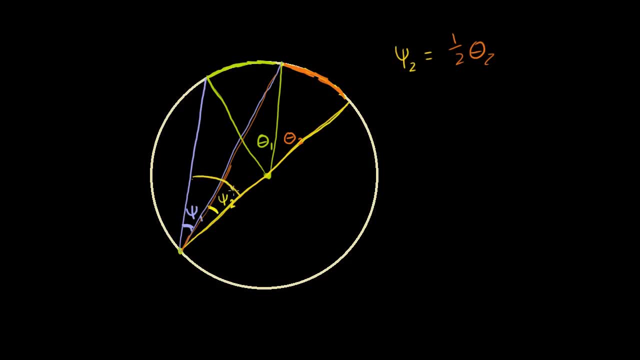 This larger angle right here: Psi 1 plus psi 2, right, That larger angle is psi 1 plus psi 2.. Once again, this subtends This entire arc right here. So it's going to be, and it has a diameter as one of the chords.